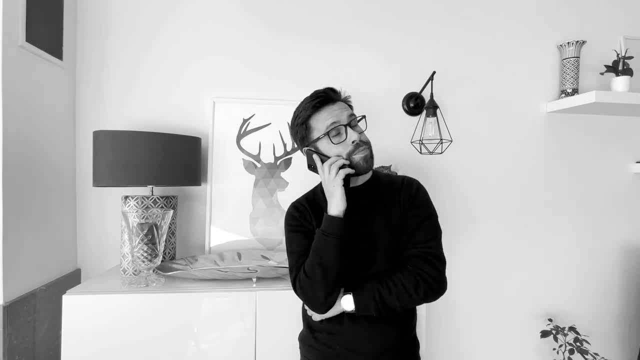 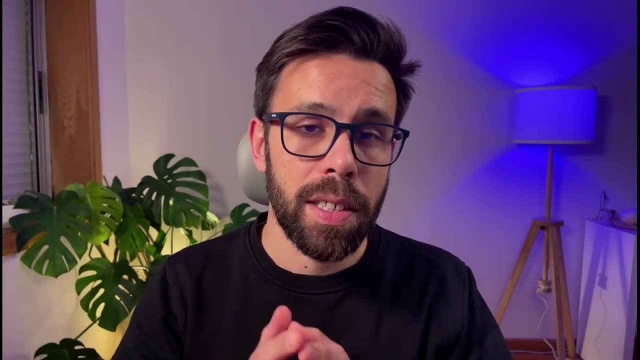 When you call your support line, your call may go through multiple persons until you finally get your problem sorted out. That is the chain of responsibility in action in the real world. You may be familiar with it if you have been using ASPNET. Chain of responsibility is a. 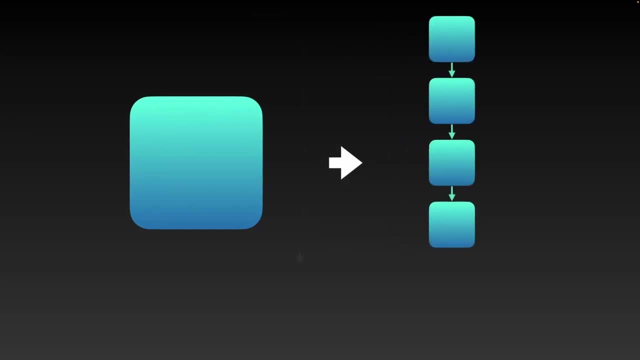 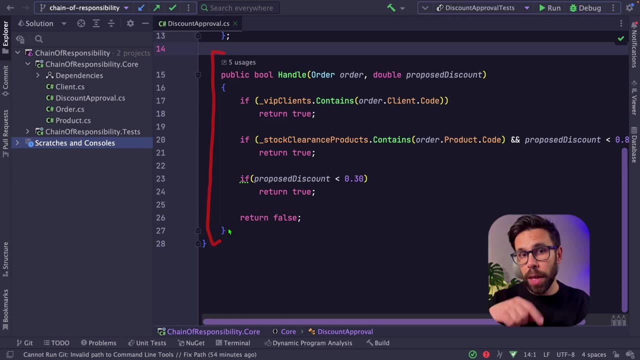 behavioral design pattern that can be really useful if you want to refactor your code by decoupling and segregating responsibilities. This is the method that we'll be refactoring today, And this is a small example where applying the chain of responsibility can lead you to better. 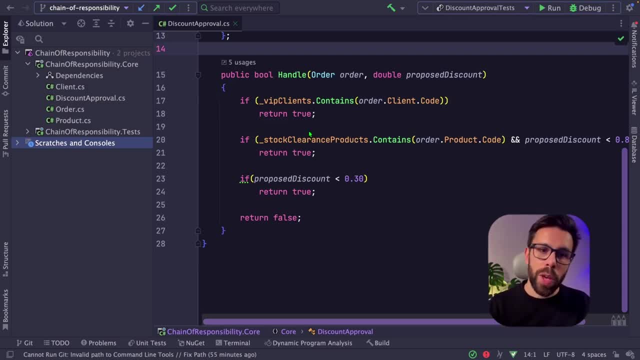 and maintainable software. So what does this thing is doing? We have here, basically, a simple function that has the responsibility of finding if, for a given order- from the order we will know- products, clients, total amount- we can give it a given discount. 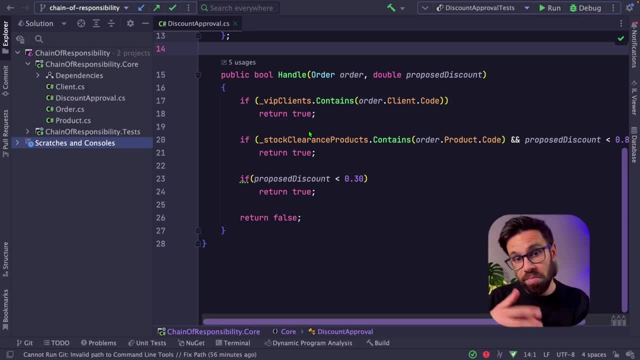 So you can imagine your sales team using this function under a given screen on your application. This is a simple example, but you can imagine what will happen when this business keeps growing and then you start bringing more discount rules on top of it and you keep updating this method and things start to get. 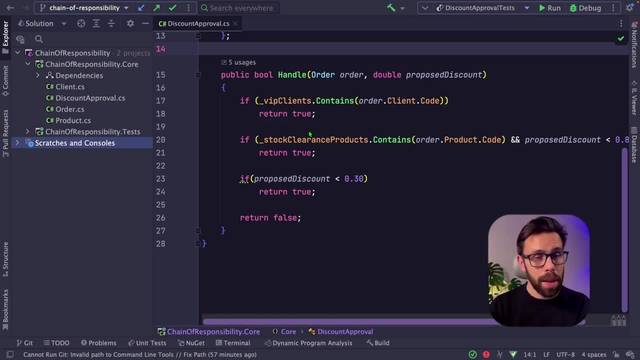 really messy. you get to a point where this class has too many responsibilities is hard to maintain. everyone is afraid of touching it. you see what will happen and why. the chain of responsibility is a good design pattern for this case, because it will help us segregate the responsibilities while 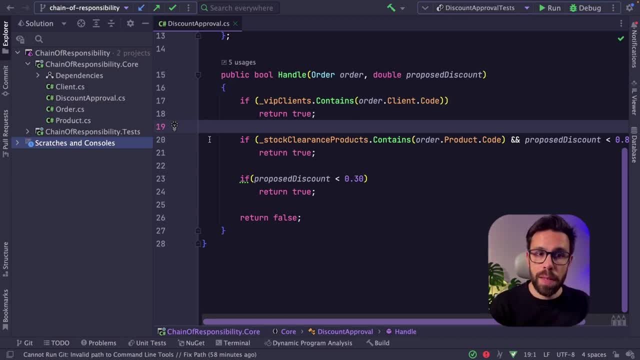 we keep the system decoupled from the consumers of this discount approval engine. other key aspect to know that the chain of responsibility is a good fit for this case is that, as you can see, there's a given order on the rule. so first i check if it's one of my vip clients, then i will check if the 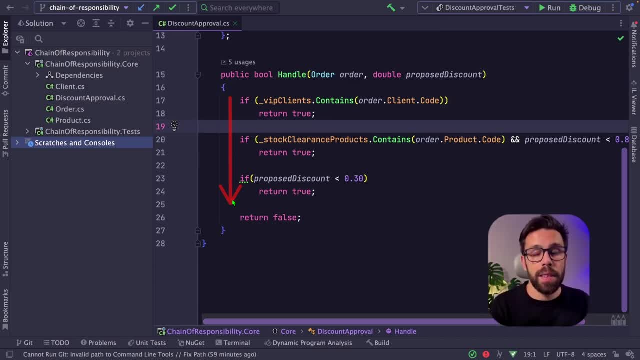 product is listed under stock clearance and the discount is below a given value. then, last but not least, i will check an overall discount rule and while i'm doing this thing in order, you can also see that the discount is below a given value and the discount is below a given value. and then 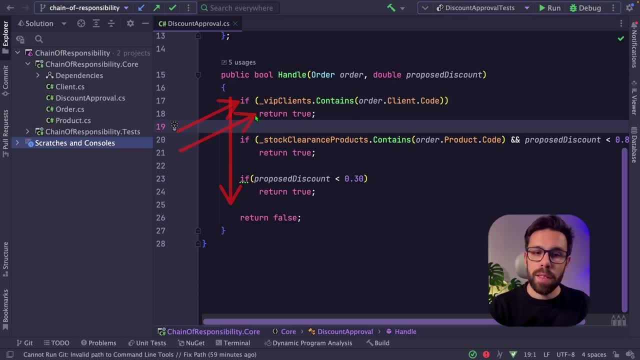 while i'm doing this thing in order, you can also see that the discount is below a given value. and then, while i'm doing this thing in order, you can also see that the discount is below a given value. and every time that i check a given rule, i may return and break the cycle, so i don't go to the next rule. 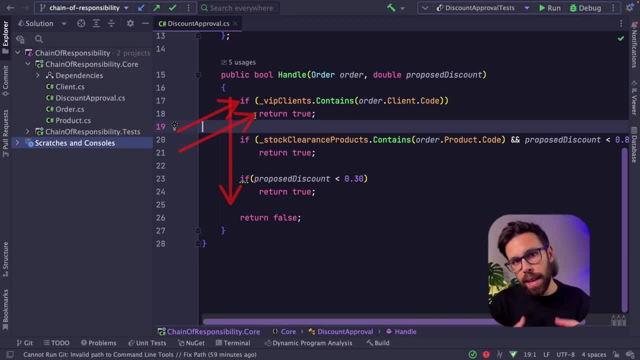 or i keep going to the next one, and this is basically the idea of the chain of responsibility: each handler will do his job and then he will delegate the request to the next one. so let's see how we can refactor this before we start to refactor. just to let you know that we have a set. 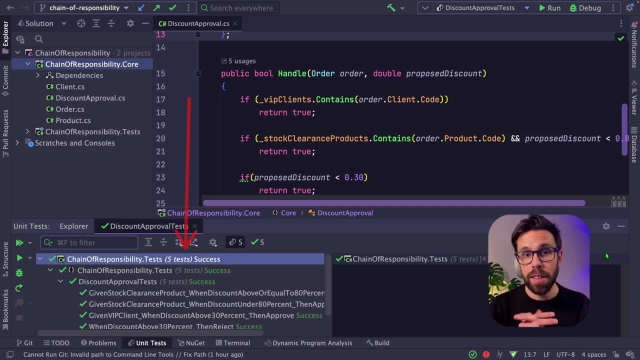 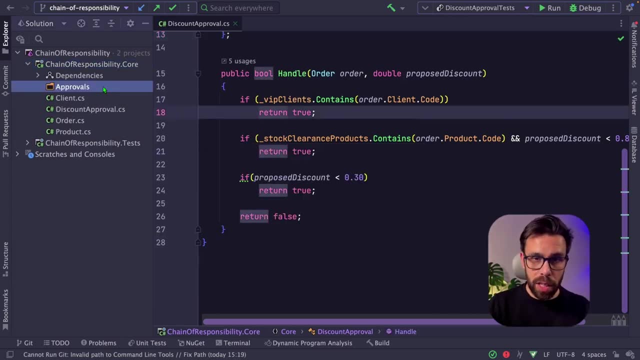 of tests that will guide our refactoring, to make sure that you didn't break anything. so the first thing that i will do is create a folder approval. i will keep all the source code regarding this chain of responsibility inside of these approvals so it's easy for you, as a patron, to grab the source code and see what it's doing. first thing, 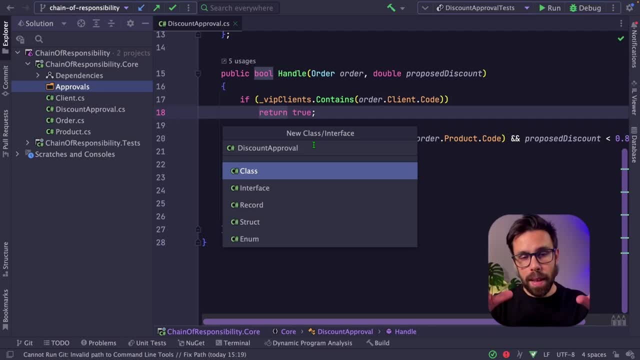 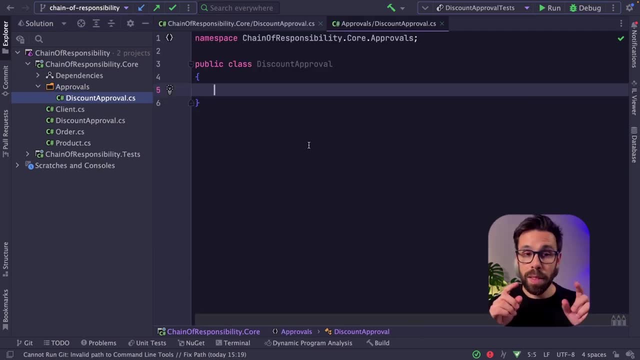 that we need to have our chain of responsibility is having our base class that will orchestrate the request and will define the guideline for the ones implementing it. i will name it: discount approval. i'm using the same naming under a different namespace, just to show you this without. 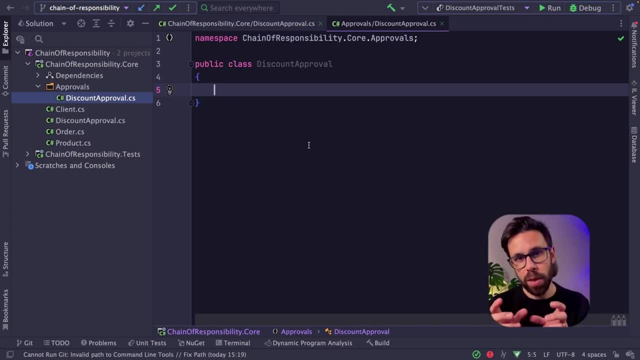 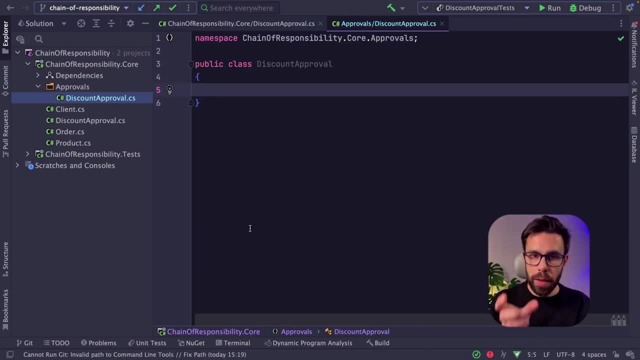 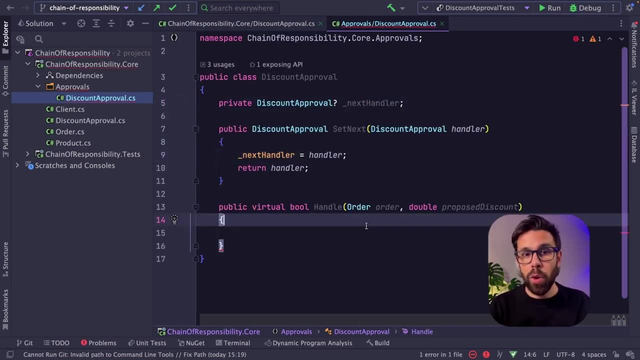 class is a method that will be responsible to keep the next element on the chain, so let's create one that will be the set. next, we need a field to store it. let's set it. and now we add another method that will be the handle of this request. so we will receive the order and propose discount, since this 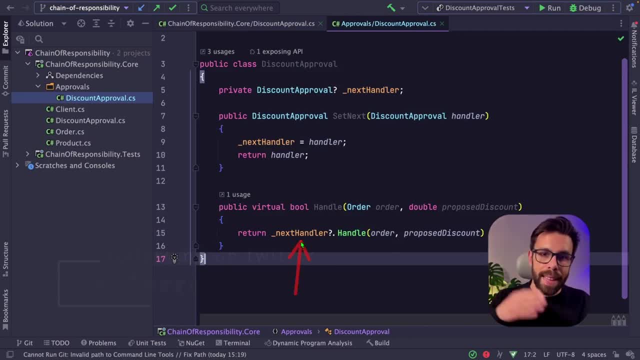 one is our base class. let's define that. if i have a next element on the chain, let's handle that one. otherwise let's return false. so what does that mean? it means that when the implementations of this discount approval are executing, if they have something next they will delegate to the next one. otherwise, it means 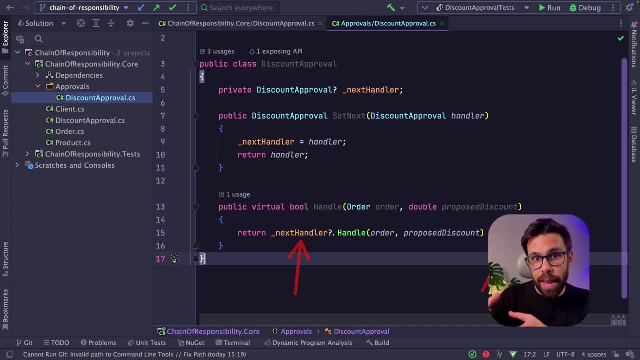 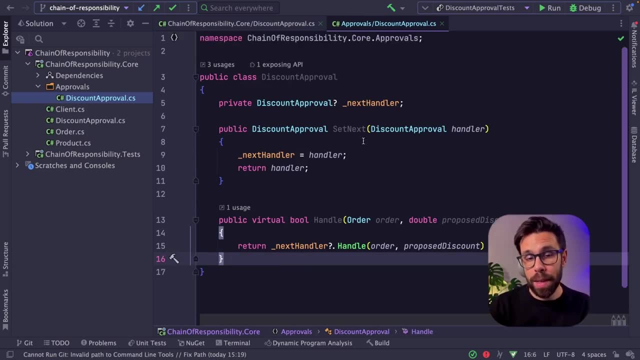 that we reach the end. so if we are in the end and we didn't return yet as true, it means that the discount is not approved. now that we have our base class, let's start to implement the rules. if we look into the old source code, we can see here three rules, and let's start by the one for the vip. 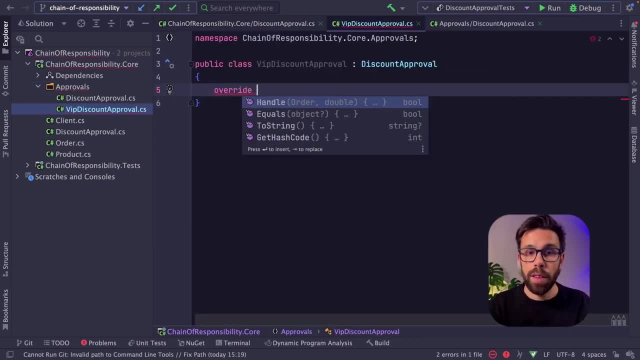 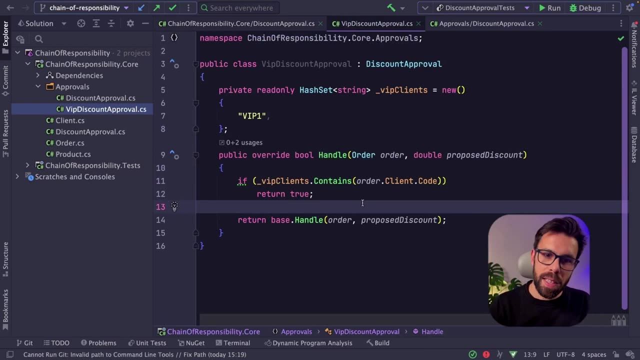 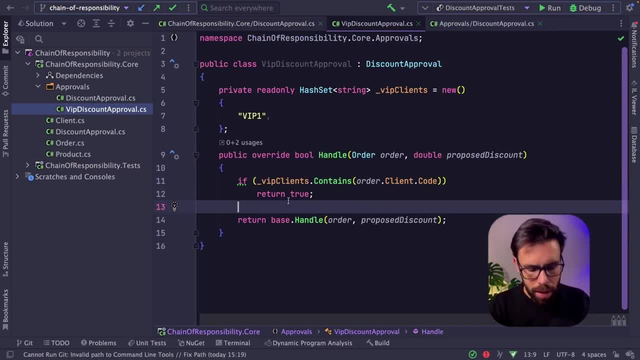 when this element on the chain executes. what will happen is that i will check my rule. i will return and break the chain if i match the rule, so the discount is approved. otherwise i will ask the base class to delegate this execution to the next time. so i'm not coupled to the new one. i'm going to 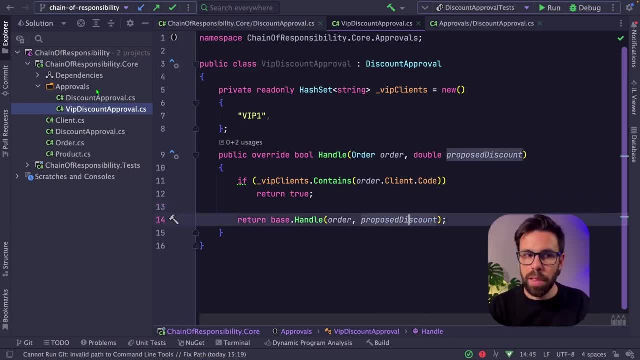 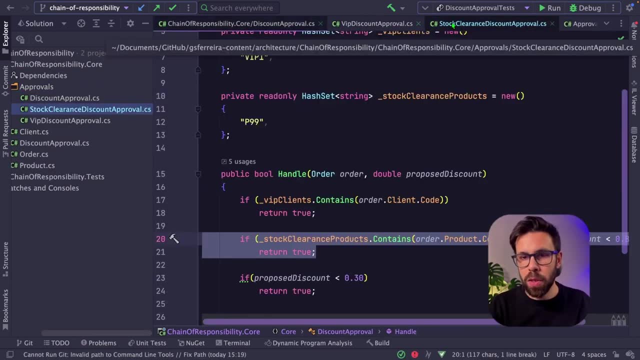 couple to the next handler and he also doesn't know me. let's implement the other rules. add one for the stock clearance. once again the same idea. override the base class and copy the source code that matters for that rule into your new handler. add my last rule: override the base class, grab the. 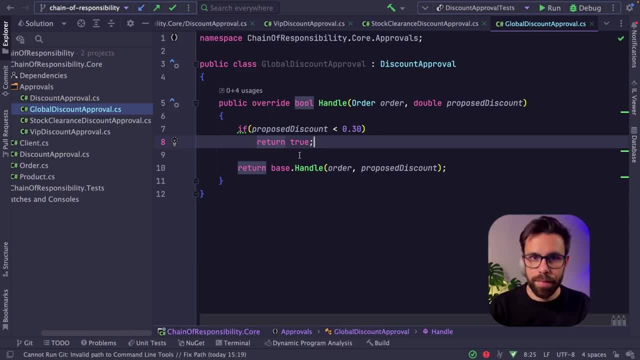 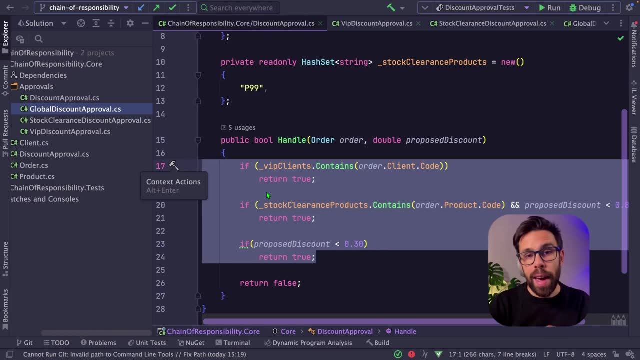 source code from the old implementation into there and it's done. now all those three rules are in individual elements of the chain, so i have segregated the responsibilities, so the next step is seeing how to execute them. to do that, what i'll be doing first is removing the old approach. 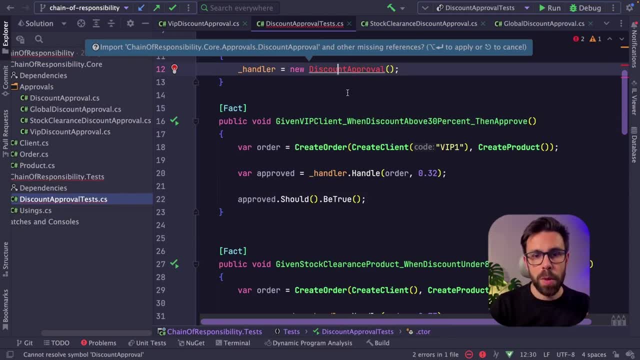 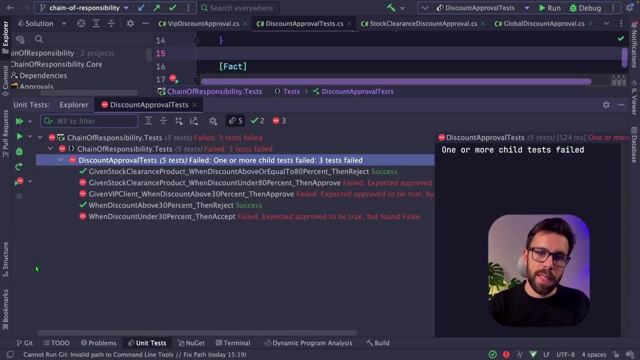 delete the old file. now my tests are complaining, but since i'm using the same naming under a different namespace, it's easy fix. let me show you what happens. if i execute the tests now. you can see that three of my tests are failing, but i have two that are green. why? because if you look into 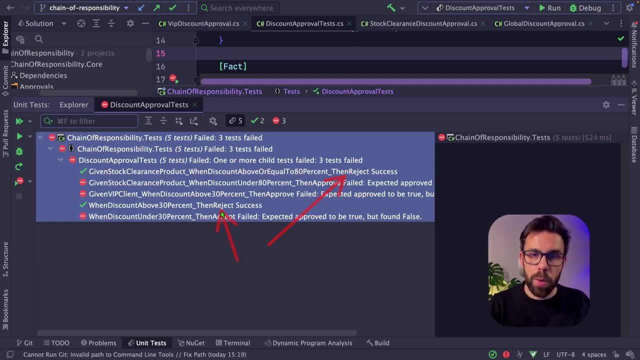 them. you will notice that both of them are regarding the reject scenario and since on my chain, when i don't have the old approach, i'm going to remove the old approach and then i'm going to create another one later on with the saga and throw it in the old approach. so i plug in for a delayed 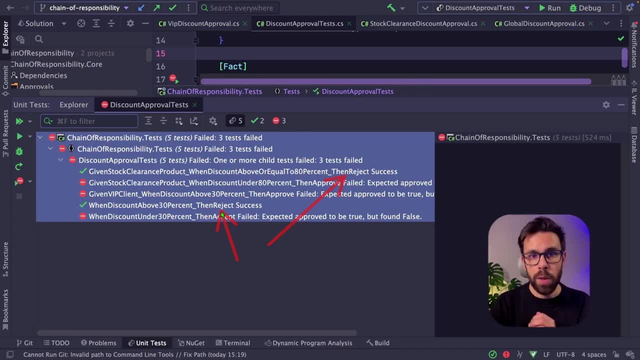 случай. look and see that both very true. now that i'm out of it, i'm not breaking anything. so after resetting it that way, i can check which dialogs are still green and i can change that from the old approach to the old approach, and certainly in my ownμέ礼도, like we talked about. 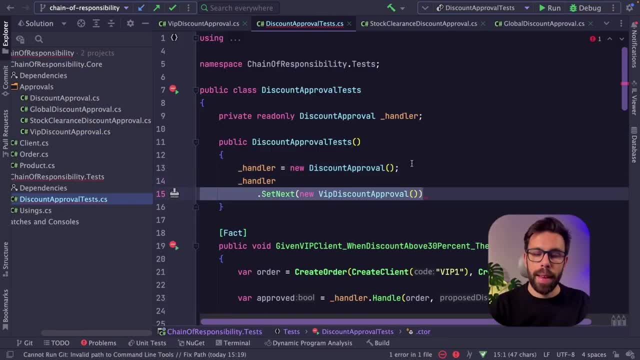 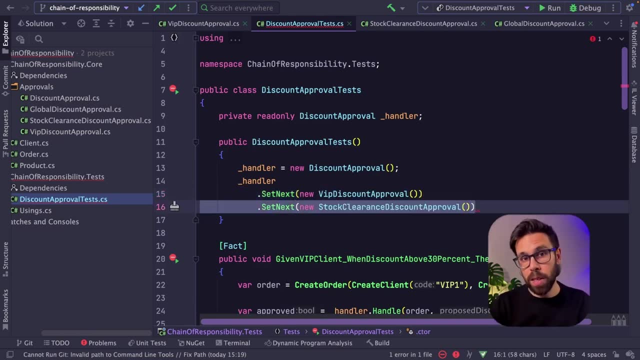 in this get酒 Ace story. we sent it to one of my bed paste filters and that's the method that information we will use. today. if we talk about database Norway, we use customers and a website. we will set up our own database, as you can see it here, this virtue of, rather than just good, easy search. 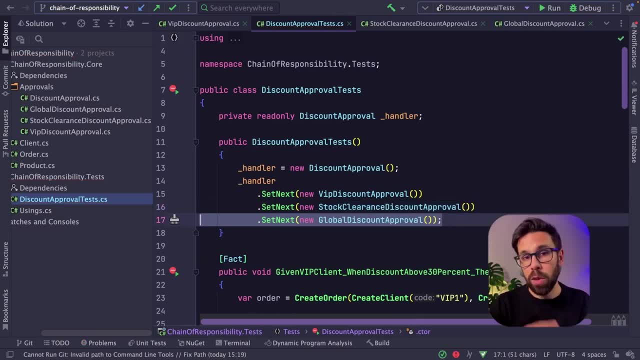 we have here backbone that is used to set this % to is using international chains and we always code this shelf on this database to check that alpha and foreign Labor чтобы to call this value. What this means is that now it's quite simple to introduce new entries here on this chain.